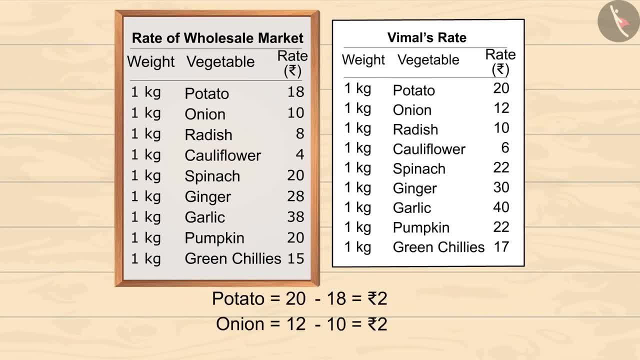 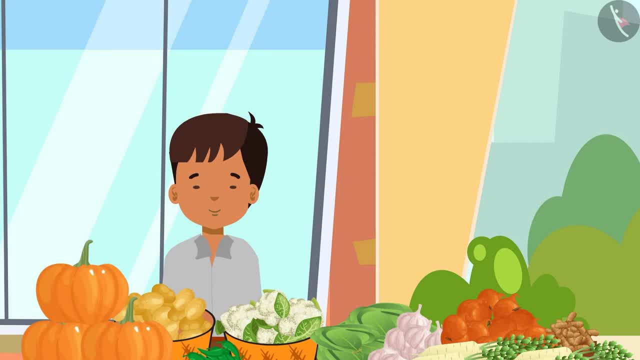 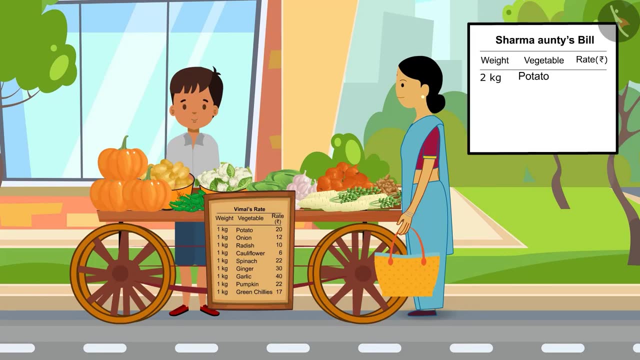 increased the prices of all the vegetables by two rupees. this extra money is Vimal's daily earnings. oh, let's see Sharma aunty is buying some vegetables from him. she bought two kgs of potatoes, 1 kg of onions, 1.5 kg of radish, 1.5 kg cauliflower and 1.5 kg of ginger. 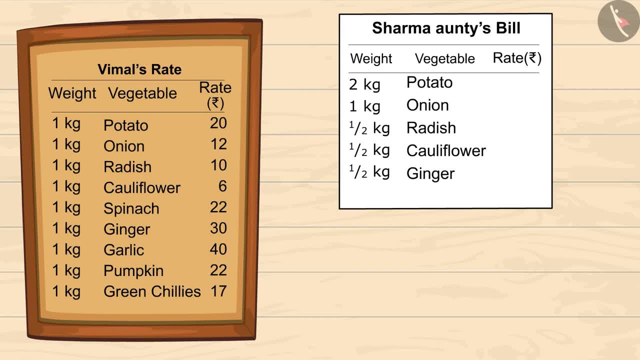 let's together find out the total price of Sharma anty- 처 phase from Vimal. you can pause the video and calculate it with the help of the mills list. according toする list, 1 kg of potato cost rupees 20, so 2 kgs will cost. to multiply by 20 means 40. 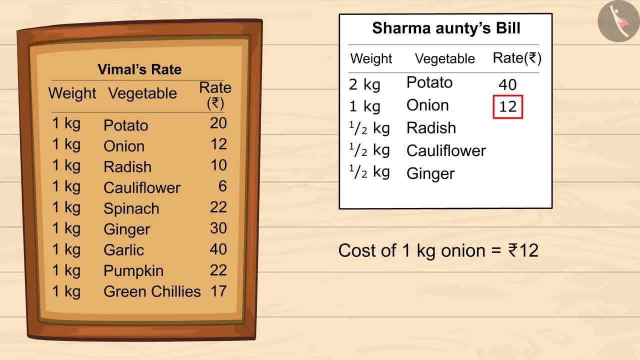 1 kg onion is 12 rupees. 1 kg radish is 10, so it is half of it. on adding 5 up to 2 times gives us 10. so cost of half a kg radish is 5 rupees. similarly, if 1 kg. 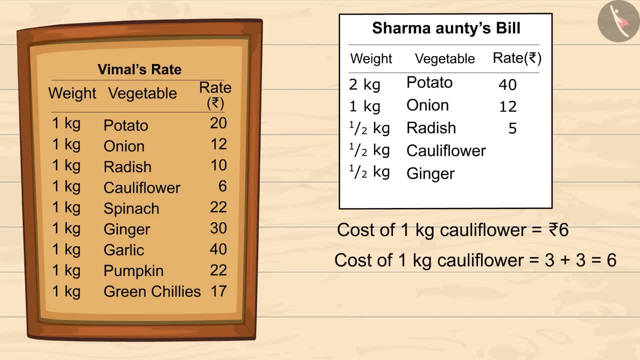 cauliflower cost 6 rupees, half of it will cost 3 rupees. now we are left with half a kg ginger means half the price of 1 kg. you can pause the video and calculate it. 1 kg ginger cost 30 rupees means half a kg ginger will cost half of. 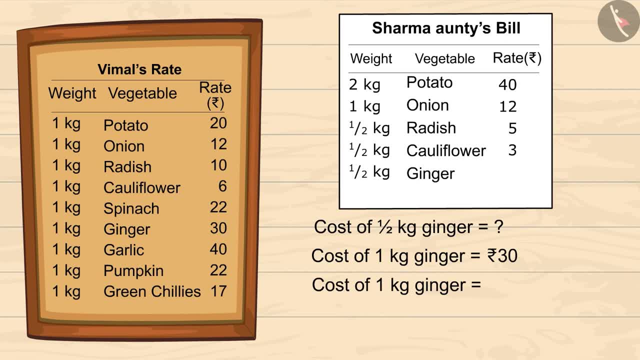 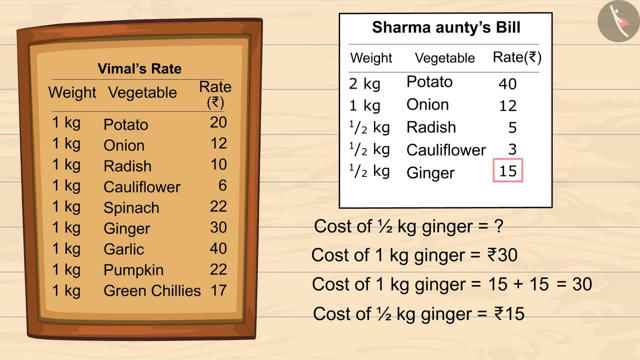 30 rupees. hmm, on dividing 30 into 2 equal halves we will get 15. so half a kg ginger will cost 15 rupees. so this is the cost of shopping done by Sharma aunty. now let's add all this to find out the total price. kids, you can pause the video to find out. 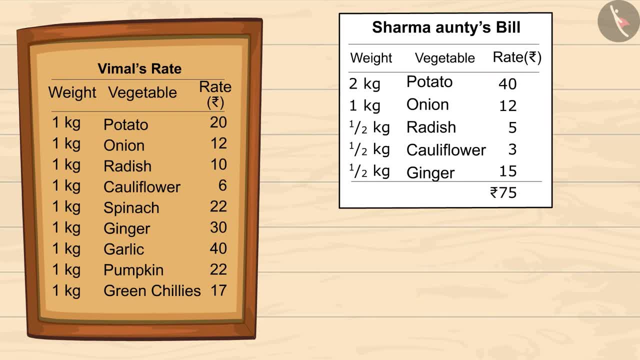 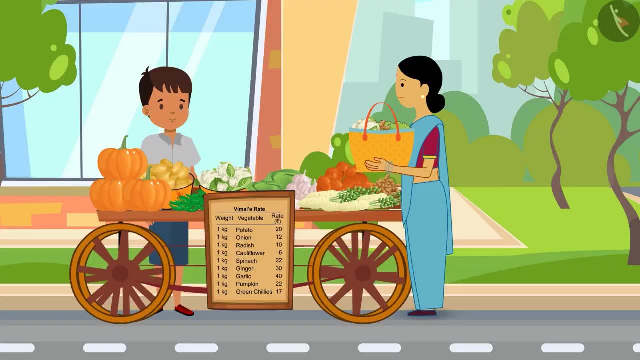 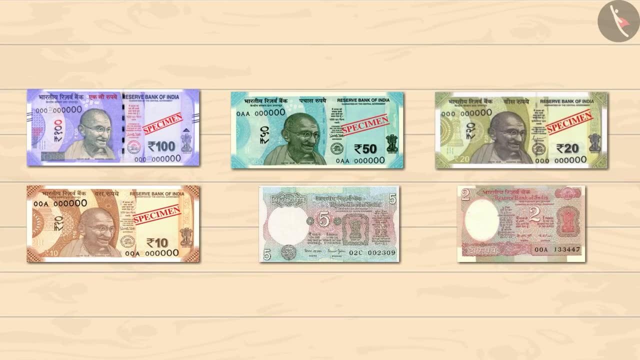 the sum. look, Vimal has already added all the numbers. is your total is also 75 rupees. Sharma aunty has to give 75 rupees to Vimal. a few notes have been placed in front of you. let's help Sharma aunty to add the total price. you can use each.